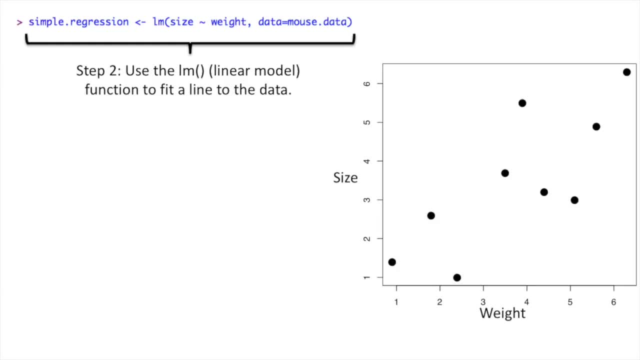 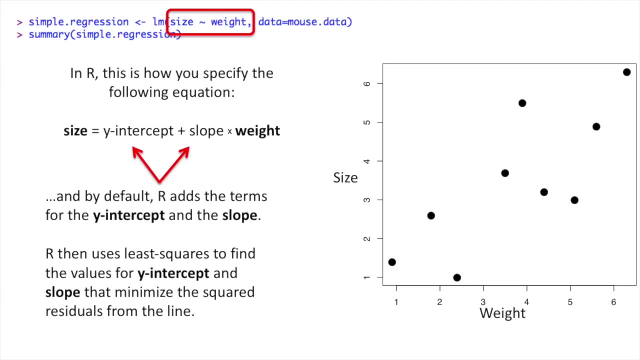 change their… …, …, …, …, …, …, …, …, …, … … and the slope that minimize the squared residuals from the line. Once we've run the linear models function and save the output in a variable called simpleregression, we can get a summary of that. 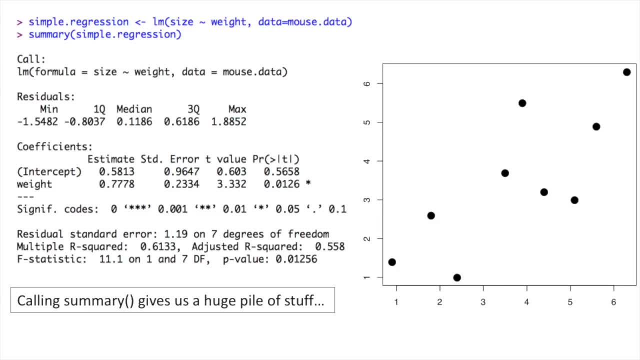 regression using the summary function. Calling the summary function on simpleregression gives us a huge pile of stuff. The most important stuff is down here, Specifically the R squared and the adjusted R squared. Multiple R squared is just another way to say R squared. by the way, 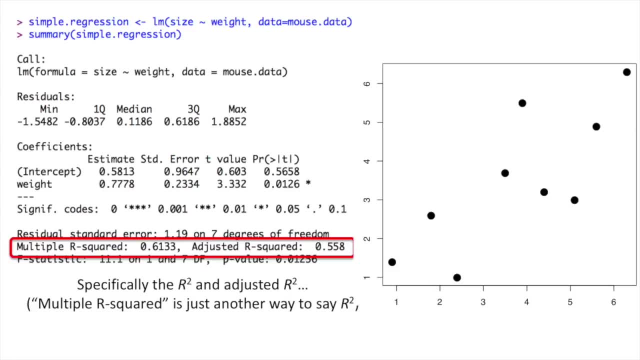 Also for simpleregression. the multiple R squared value, or just plain old R squared, is the one we're interested in. The adjusted R squared only applies when we have more complicated models. We'll use it later when we do multiple regression. There's also the p-value down here, Together the R squared. 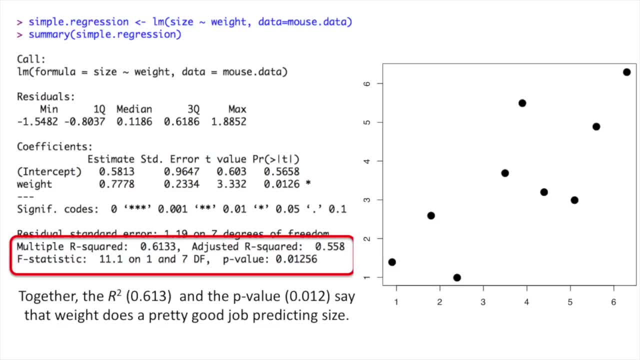 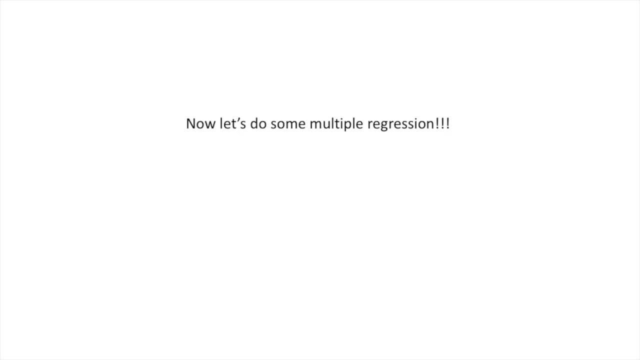 which equals 0.. 0.613, and the p-value, which equals 0.012, say that weight does a pretty good job predicting size. The last thing we want to do for our simple regression is add a line that shows the least squares fit on the graph. We do this using the AB line function. Now let's do some multiple. 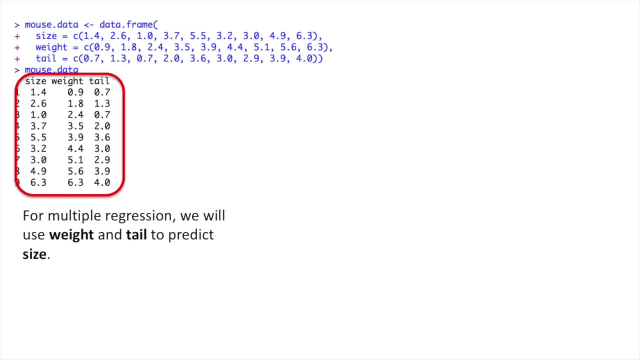 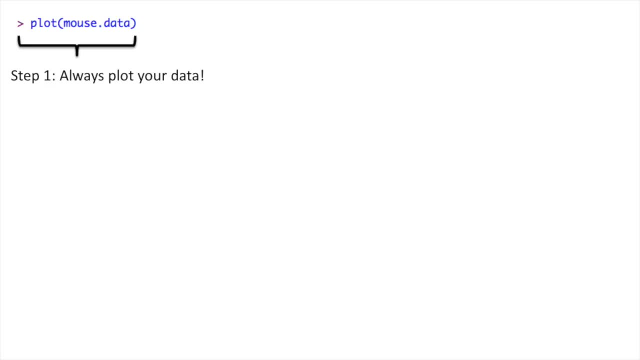 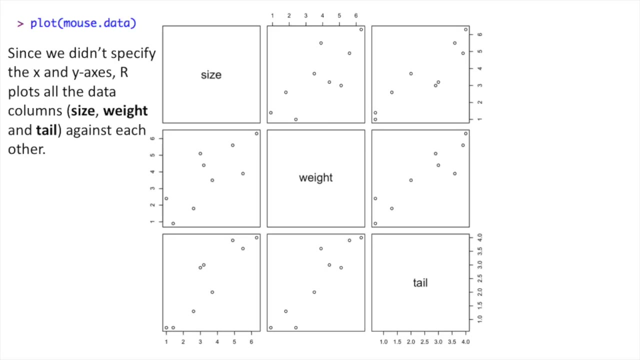 regression. For multiple regression, we will use weight and tail to predict size. Step one: always plot your data. Since we didn't specify the x and y axes, R plots all the data columns- size, weight and tail- against each other. This is super useful because it generates all the 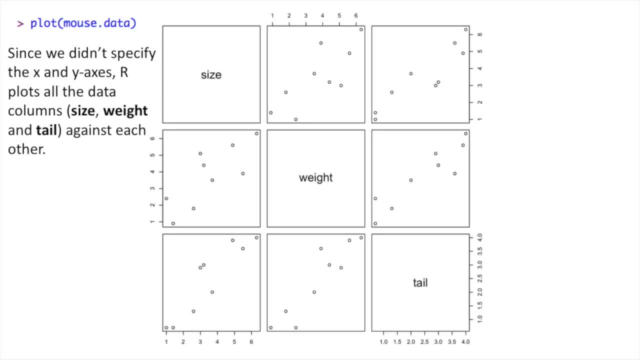 plots. we need to decide whether doing a multiple regression with this data makes sense or not. This graph plots size on the y-axis and weight on the x-axis. This is what we used before in the simple regression Down here. we have the same exact data. however, this time size is on. 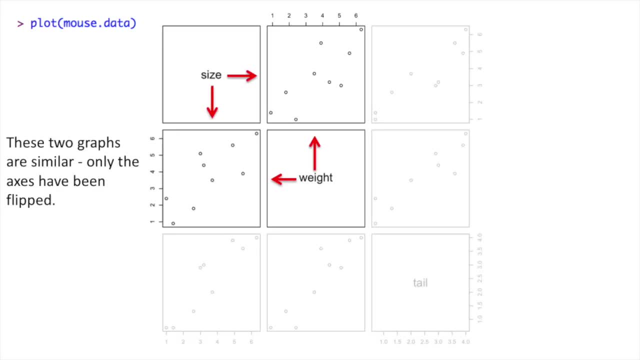 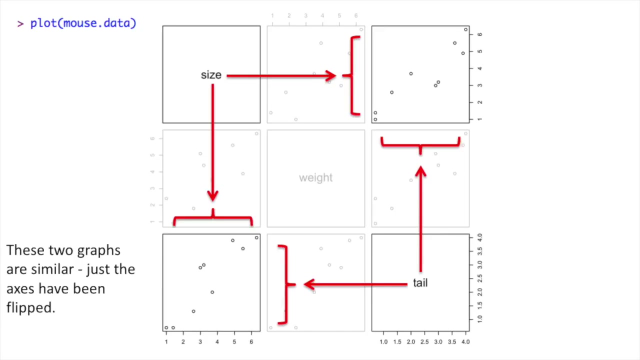 the x-axis and weight is on the y-axis. These two graphs are similar, Only the axes have been flipped. The graph in the upper right hand corner has size on the y-axis and tail on the x-axis, And in the lower left-hand corner we have another graph. 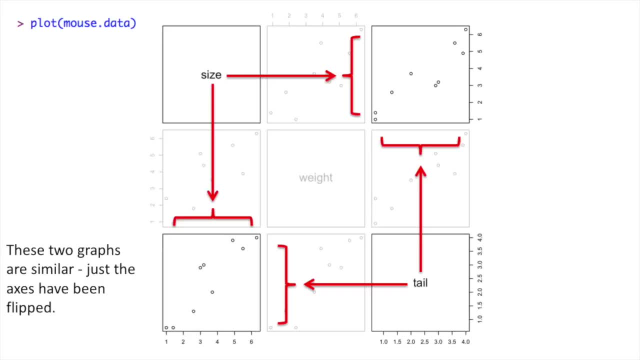 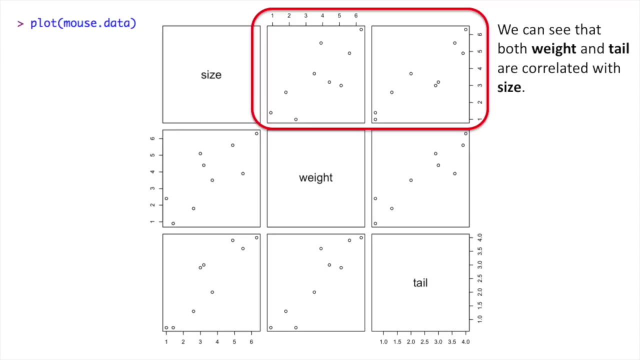 that's very similar, just the axes have been flipped. This graph has weight on the y-axis and tail on the x-axis And, just like for the other graphs, these two graphs are similar, just the axes have been flipped. We can see that both weight 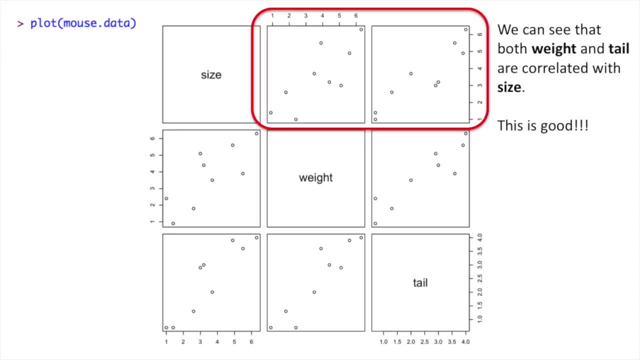 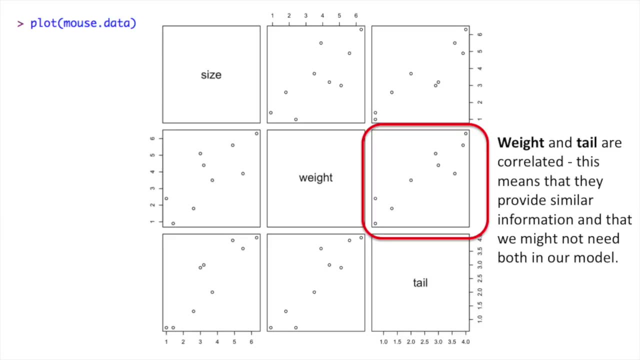 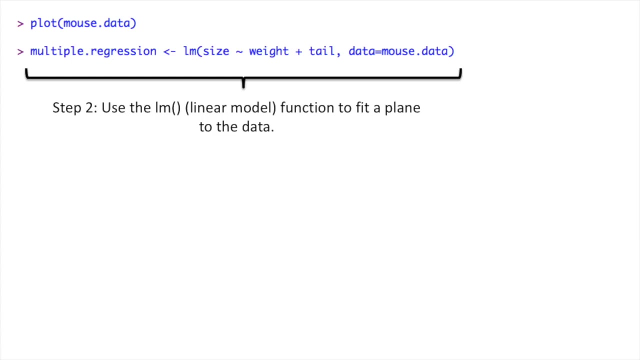 and tail are correlated with size. This is good. It means that both weight and tail are reasonable predictors for size. We can also see that weight and tail are correlated. This means they provide similar information and that we might not need both in our model. We might only need weight or tail. Step 2, use the. 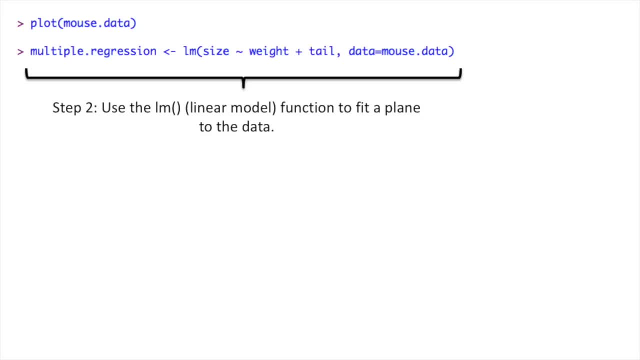 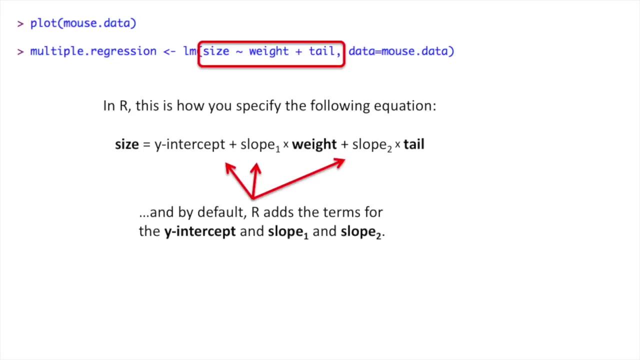 linear model function to fit a plane to the data In R. this is how you specify the following equation: Using the tilde and the plus symbols. we specify that size is predicted by weight and tail And by default, R adds the terms for the y-intercept and slope 1 and slope 2.. 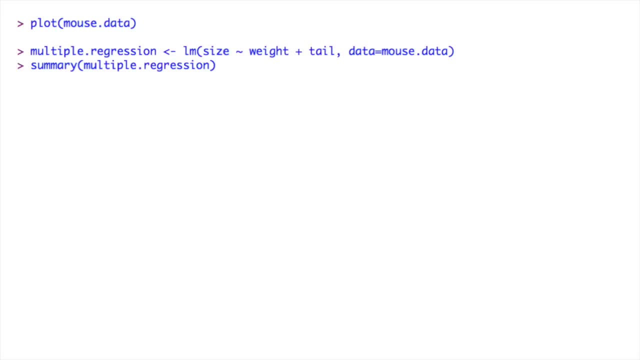 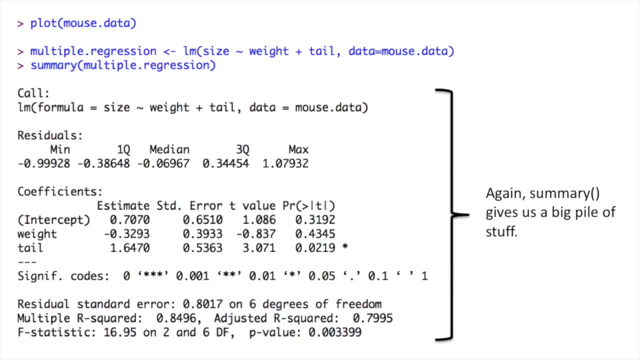 Once we've run the linear models function, we can print out a summary of the results using the summary function. Again, summary gives us a big pile of stuff. The R-squared, adjusted R-squared and the P value look good, Hooray. Note: since we're doing multiple regression, we're now more.